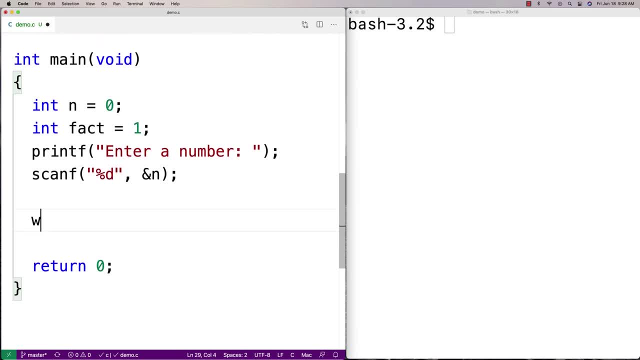 we're going to compute the factorial. So what I'm going to do is I'm going to have a loop and I'm going to say: while n is greater than or equal to 1,, run this loop and we're going to say that the factorial is equal to n times. 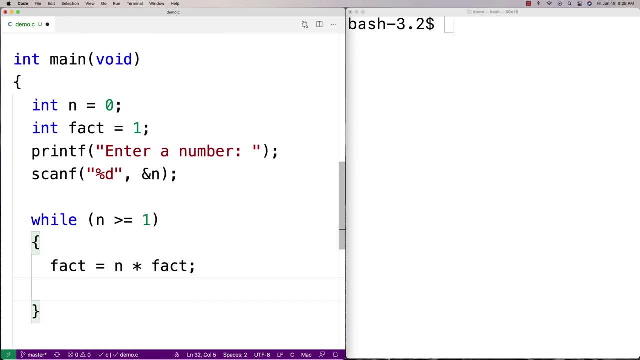 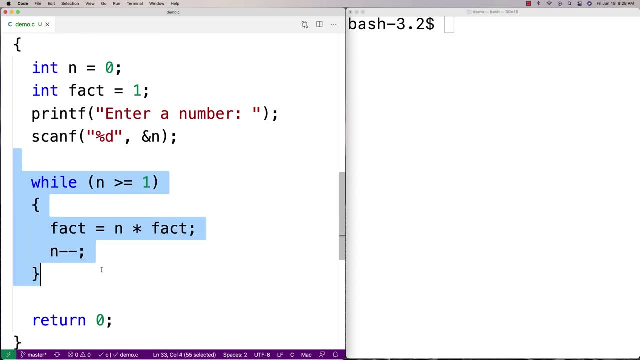 the current value of the factorial, and then we'll do n minus minus here to reduce n each time. and what we're doing here is we're carrying out this, this algorithm, in an iterative way. So we're starting off with n and multiplying it by whatever the factorial currently is, which is going to be 1.. 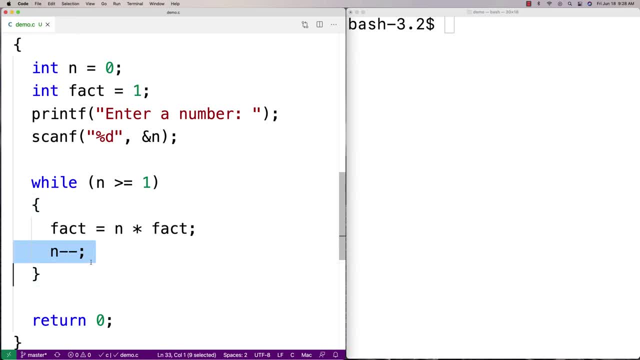 So n times 1 is just going to be n initially, right. then we subtract 1 from n. the loop is going to run again until n is greater is, until n is, you know, 0. but the loop is going to run again and then we're. 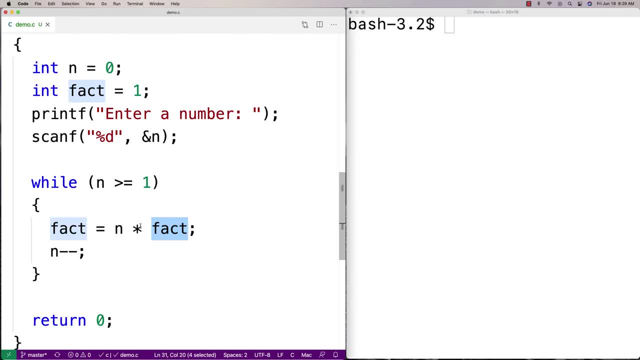 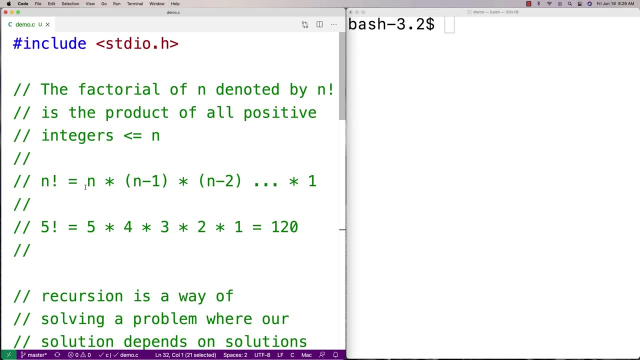 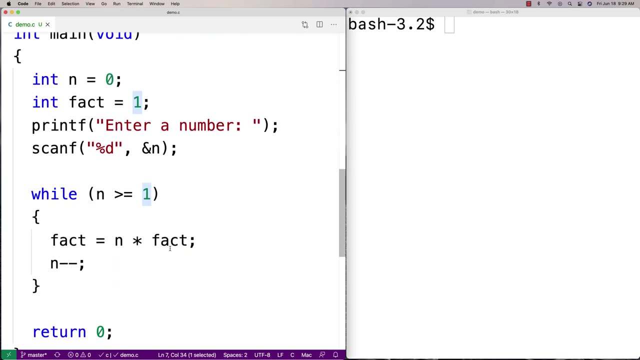 going to do n minus 1 times, whatever factorial is, which is n, and then the loop is going to run again. it'll be n minus 2 times, whatever the factorial has been so far. and so we're building up this, this result. then we're with n times ms1, times ms2, until one, once it's one. that'll be the last time, a. 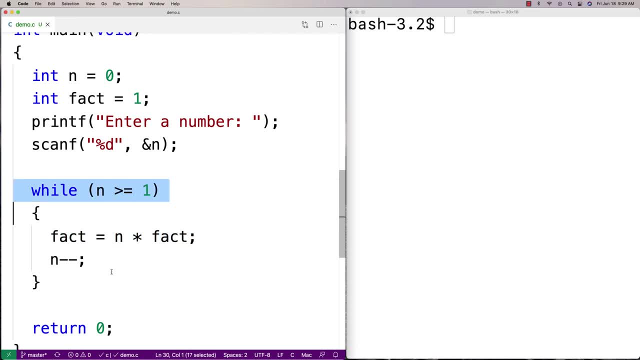 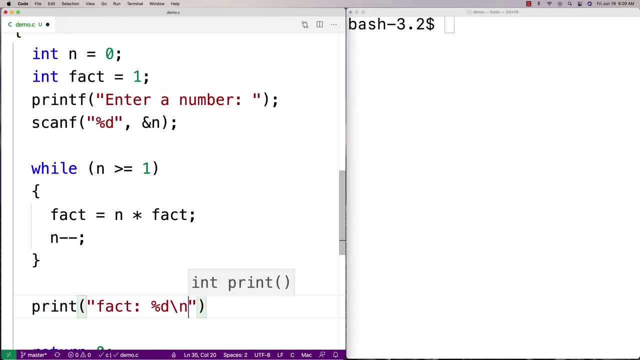 multiplication takes place and then the loop is going to, is going to terminate, and then we're done. so we can then print out the results. we could say like printf factorial is, and we could say fact there, and then we'll just compile this and give it a test. So this is like the iterative. 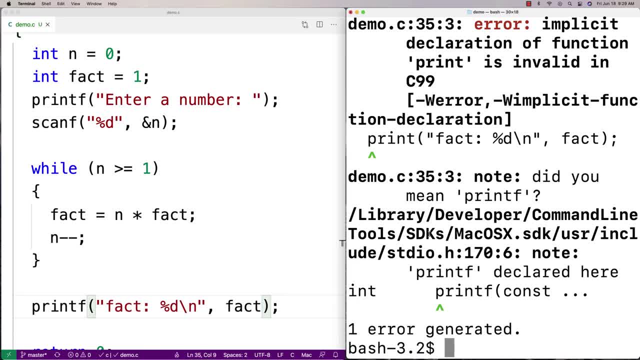 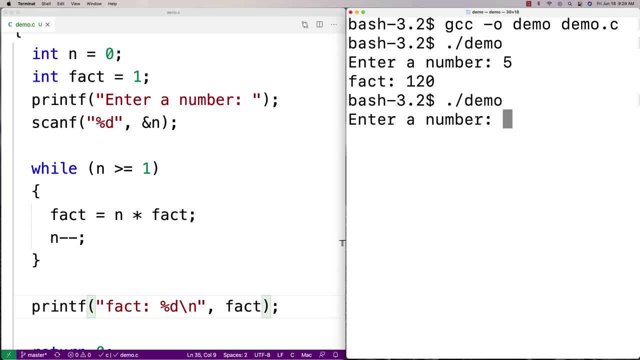 solution. this is the typical way of solving the problem. oh, I forgot the f there with the printf. so this is the typical way of solving the problem. so it says: enter a number, we'll put in 5, we get 120.. put in 10, we get a very. 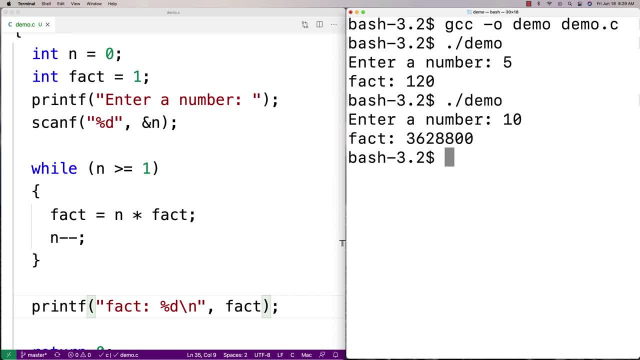 large number, so factorial explodes very quickly, but it looks like it's working correctly. so let's actually now solve this with a recursive solution. so we're going to write a function that calls itself to solve this problem, and so what I'm going to do actually is I'm actually just going to 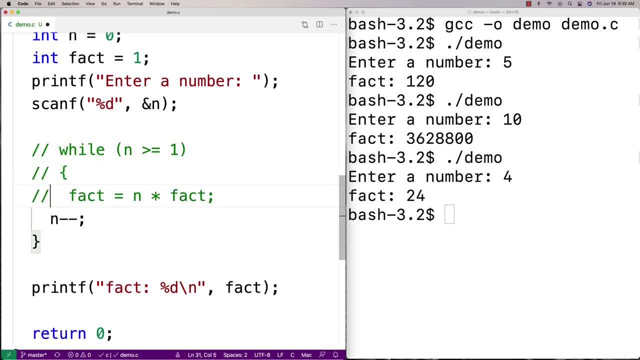 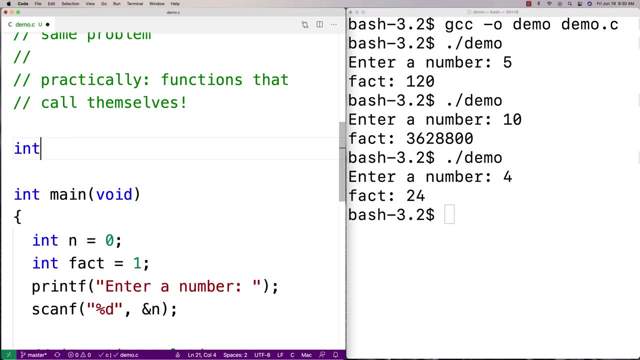 comment out this for now. so I'm going to put some comments here just to kind of, for now, get rid of this solution and we'll call this like our, our iterative solution. and now let's write a recursive solution. so I'm going to make a function that's going to compute the factorial, so I'll call it int and I'll 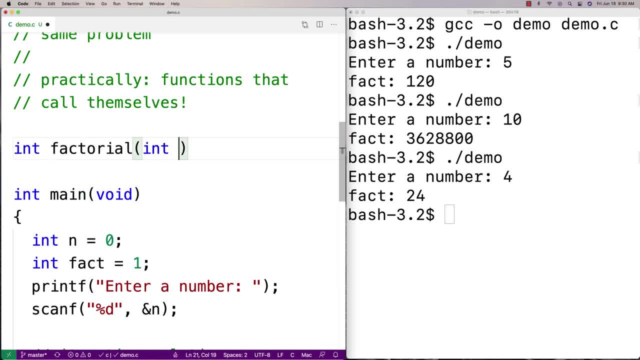 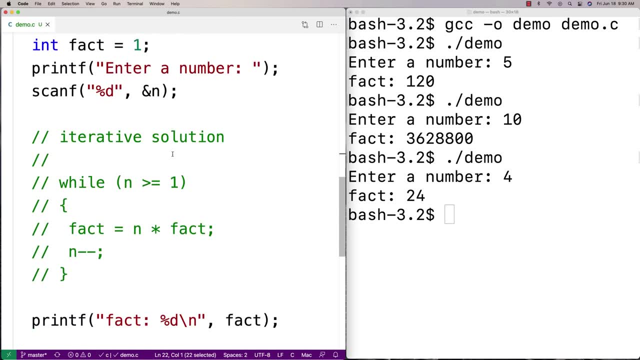 say factorial, it's going to take in a number, and we might as well call it n, and it's going to return the factorial for the number n. so let's copy this down here and then we'll make our function definition. so our function definition is actually going to be kind of short here. what we're going to, 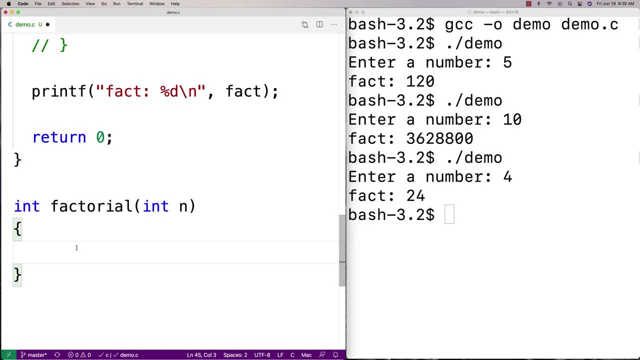 say is the factorial is going to be return factorial of n minus one and we're going to multiply n by factorial n minus one. so if you look at this here, return n times factorial n minus one. if you look at this, we've actually kind of got the structure. 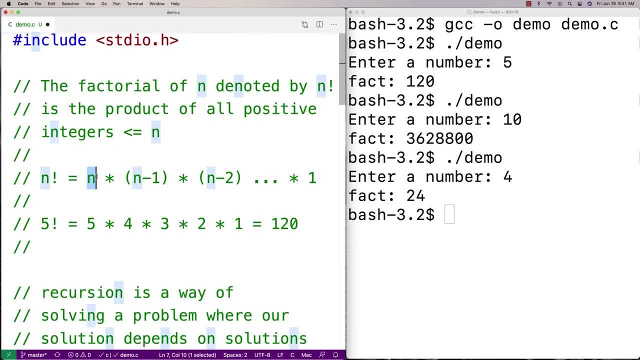 of the factorial already, because if you look at it, we've got like n times n minus one already, right. and then what's going to happen when we call factorial n minus one, when we call factorial n minus one, it's going to return n minus one times n minus two, right, and that's exactly what we want. 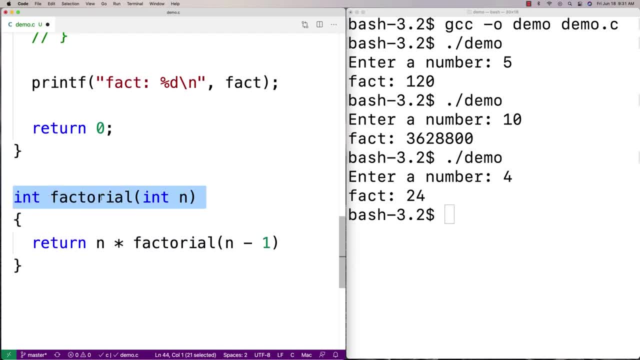 if you think about this function right here, if we recall factorial n, like let's say we call it with um with five, so we call factorial with five- what it's going to do is it's going to return five times factorial of five minus one, which is going to be what? four? right? so then, this function here, what's it going? 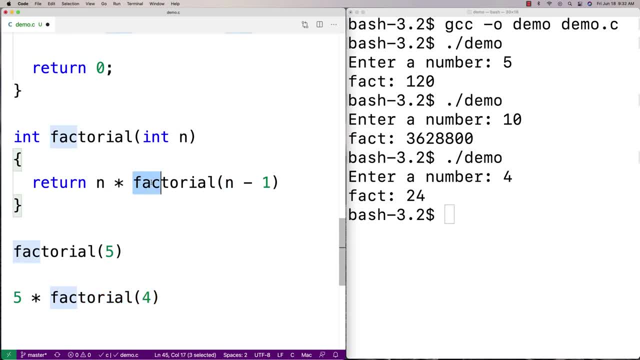 to do? it's going to return 4 times factorial of n minus 1.. so this function here is actually going to return. next, it's going to return 4 times factorial of 4 minus 1, which is going to be 3. and then, when this function runs, what's factorial 3 going to be? well, factorial 3 is going to be. 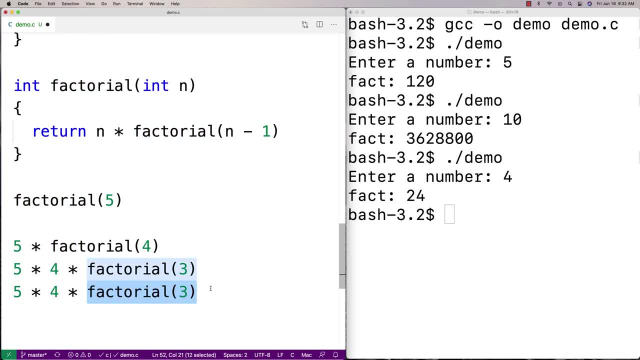 you know, 5 times 4 times 4 minus 1, three, because it's going to be three there, right Times, factorial of two, And then again, like we're going to keep going here, right? So this is going to be, you know, now it's going to. 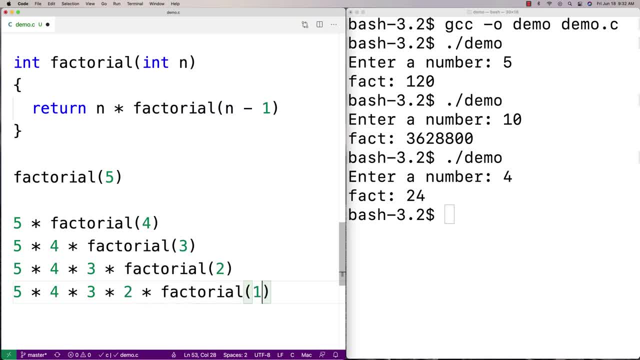 be two times factorial of one, And you can see that we're, by this having this function call itself repeatedly. it's going to keep on returning, like you know, five times. Okay, what's the next number? It's going to return four times. Okay, what's the next number? Three times, And it's. 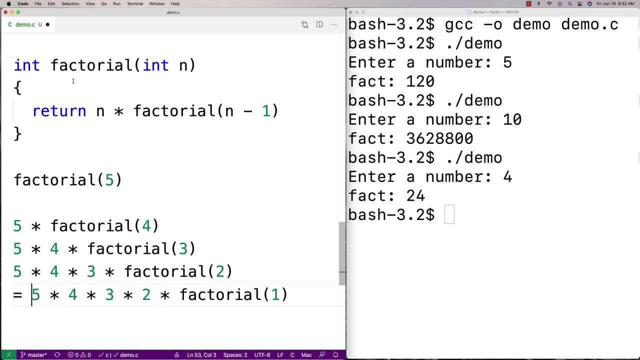 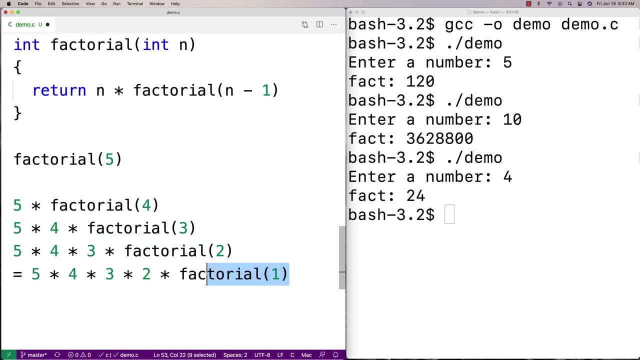 going to actually build up the result so that the function will eventually return with the result. Now the only problem is is look at this here: factorial one: When we get down to one, do we still want to return? factorial of n minus one: Does that still make sense at that point? 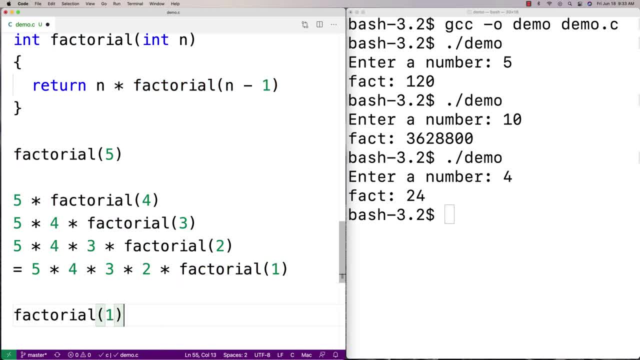 Because factorial of one would be what Be one times factorial of zero? The way we have it defined right now would be one times factorial of zero. And then what Factorial, if zero is going to return? you know, zero times factorial of, you know, I guess, negative one at. 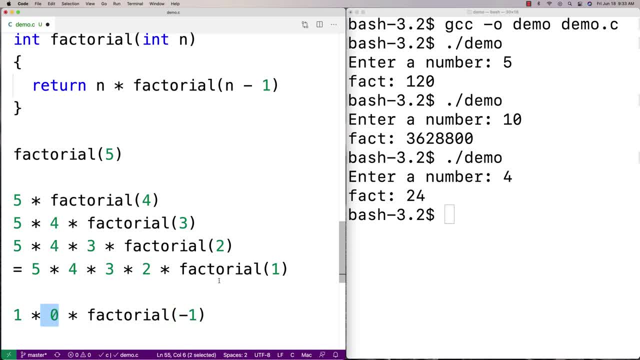 this point? right? This is starting to look bad. now We're going to multiply something by zero. This is this. this. we need to do something here, right? This, this. it doesn't make sense to keep on recursively calling the function at this point. This is where we want to stop, Because we only 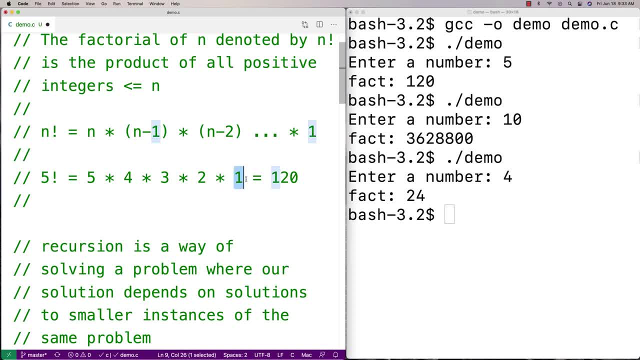 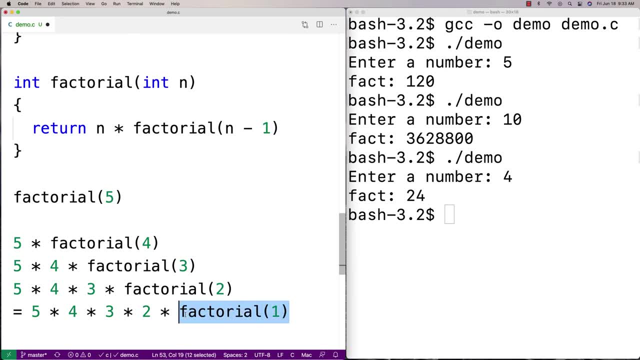 want to go until one. Once we reach one, we want to kind of stop doing recursion. We want to stop it. So this, this point where we stop recursion, we call this a base case. We call that a base case, And that's where we want to stop. 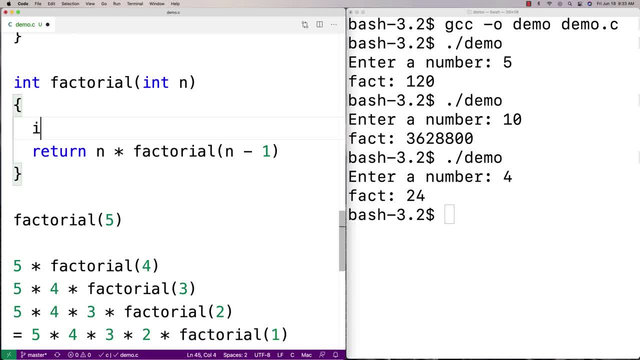 using recursion. So what we're actually going to do here is we're going to say if n is equal to one, we're going to return one And we're going to stop the recursion at that point. So this is our base case. we're saying, We're saying if n is equal to one. that's the point at which we're done. Just. 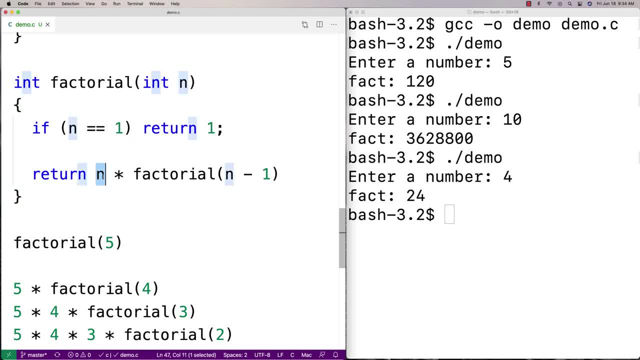 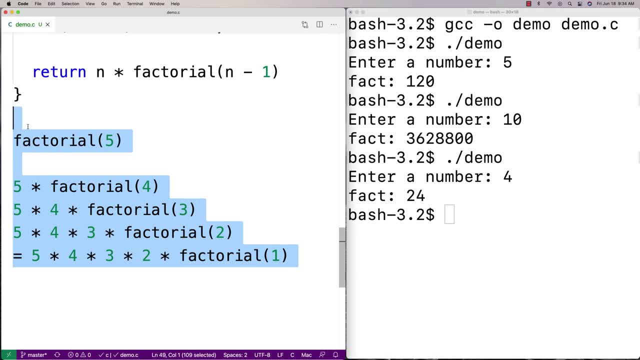 return one, Don't actually return like the number, and call the function again with the smaller number, Because at that point we want to stop, And so we can give this function now a try. Let's just see how it works. So I'm going to now call. 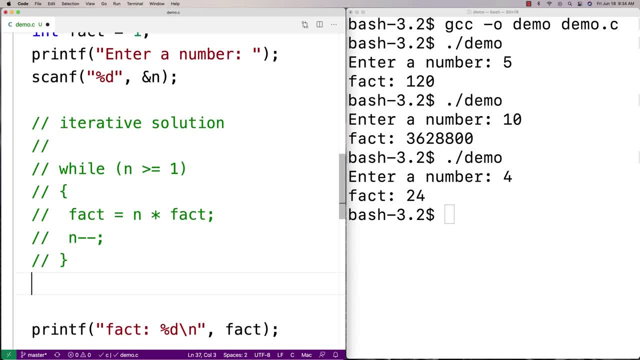 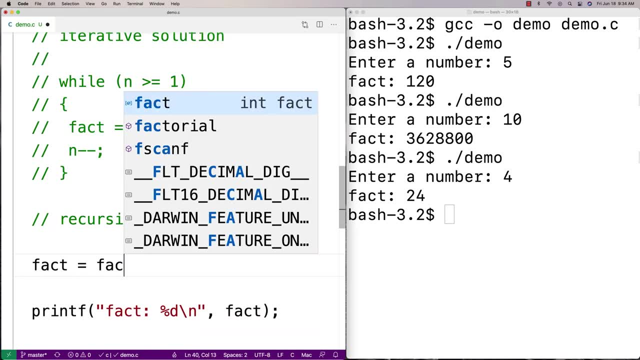 the function instead. So instead of this iterative solution, we're going to have a recursive solution. And what the recursive solution is going to do is we're just going to say: fact is equal to factorial, And we'll say: we call it with. we call it with the number n. 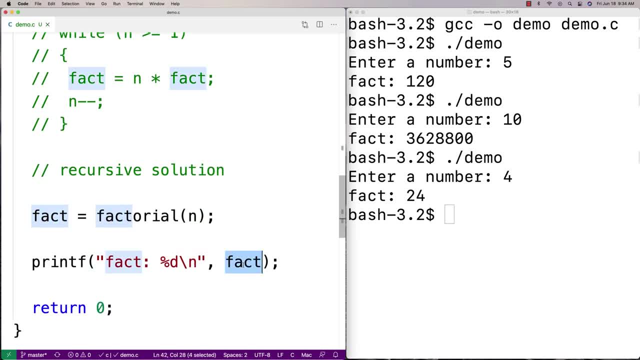 So we're going to call factorial with the number n, store the results into fact and then we're going to print it out. Okay, Let's give this a shot now And we'll just kind of: yeah, we'll focus on this part of the code. 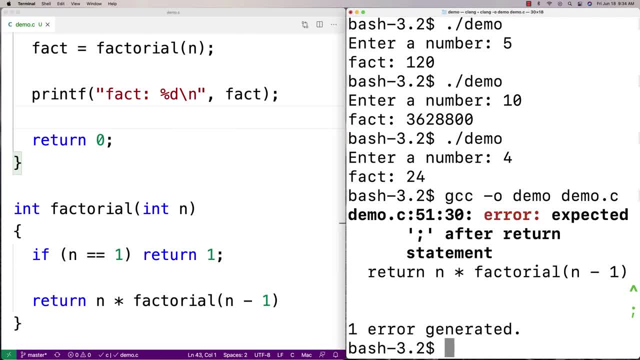 here, just because that's the interesting part for what we're doing here. And what did I do? Oh, I forgot a semicolon. Forgot a semicolon. If you were watching this video the whole time, you're probably like he forgot that semicolon. That's funny. All right, We'll clear this. 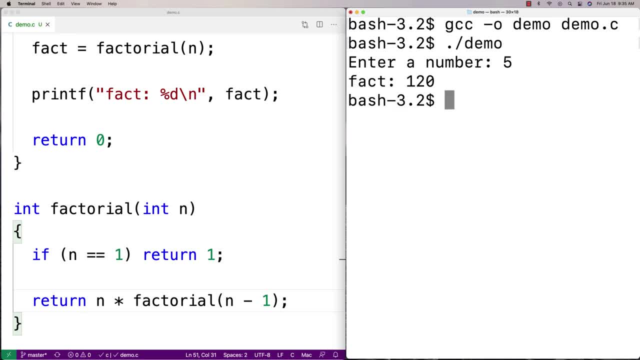 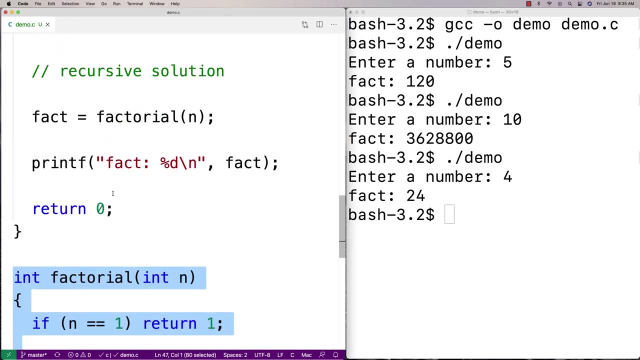 run this here and enter a number. We'll say five. We get 120.. Enter number 10.. We get the right number. again, Enter number four- Again the right number. So our solution is working And it's producing the same numbers as this iterative solution, And so we're happy. 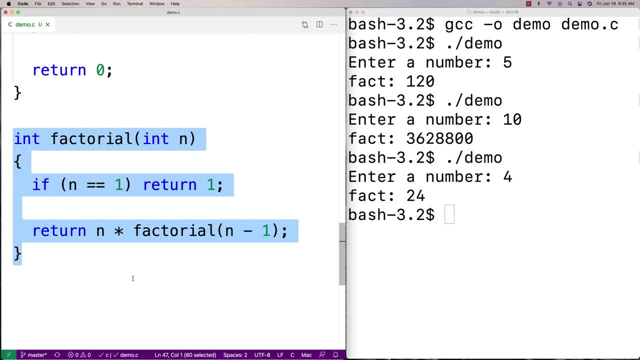 with it. Now, the kind of the advantage of recursion really is that it's expressing the problem, or at least one of the advantages of recursion is that it's expressing the problem in a way that's very similar to the mathematics of the problem. So if you look at this here, 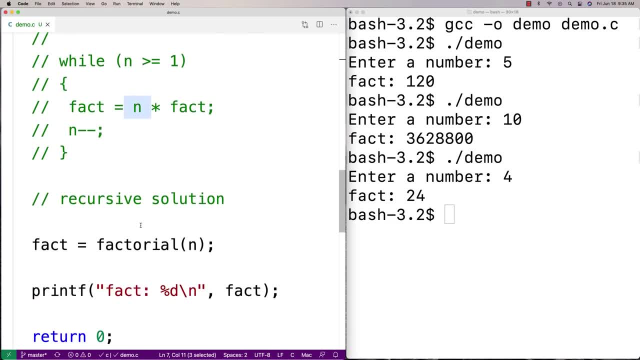 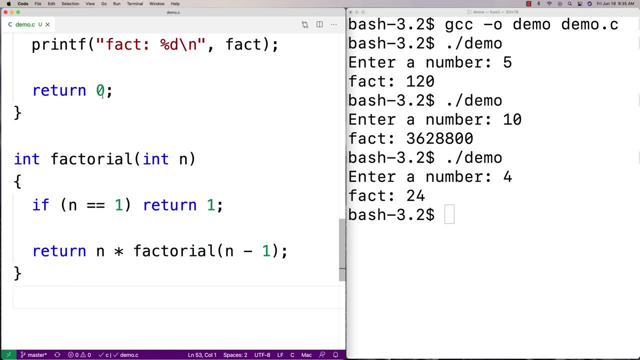 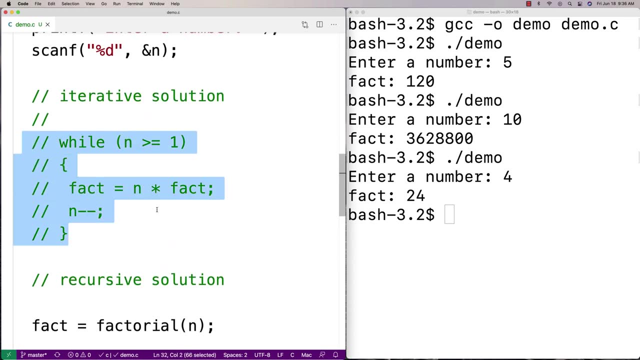 like n times n minus one times n minus two. if you look at our solution, there's a very clear relationship and mapping between our solution and the actual mathematical description of the problem we're solving, Whereas if you look at this solution here it's a little bit. 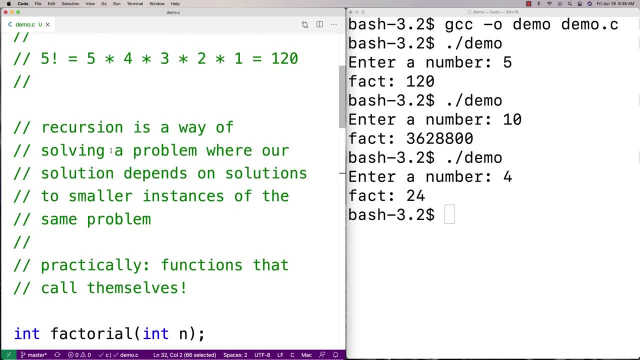 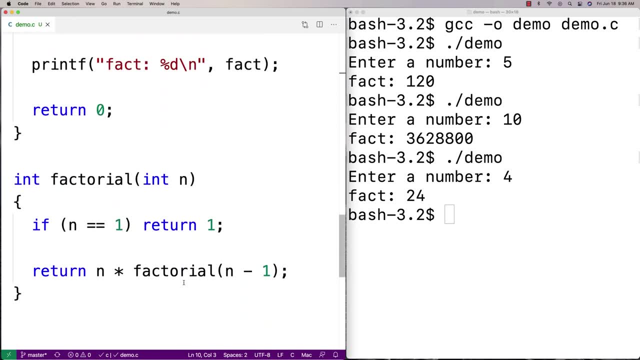 less clear what the relationship is between this solution and this mathematical description of the problem. So, recursion, using it as a tool to solve problems, it can often be sort of a more elegant, straightforward, easier to understand way of solving problems. Now, that's not always. 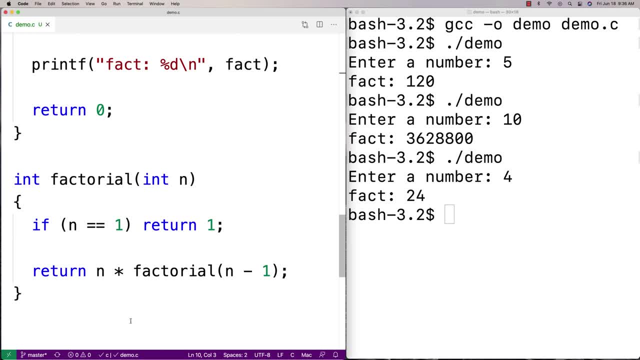 the case. It's not always the case. It's not always the case. It's not always the case. Sometimes, recursion can actually make things more confusing, And recursion can also have some performance issues as well, because you've got a function that's calling itself. 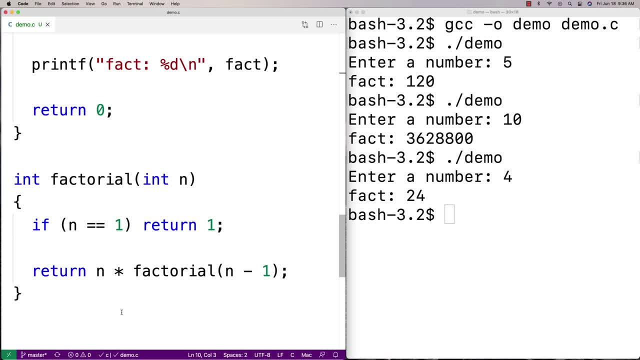 If you have a function that calls itself many, many, many, many, many times, that can actually lead to issues When your computer essentially runs out of the ability to keep having the function call itself. it's actually possible to reach a limit where a 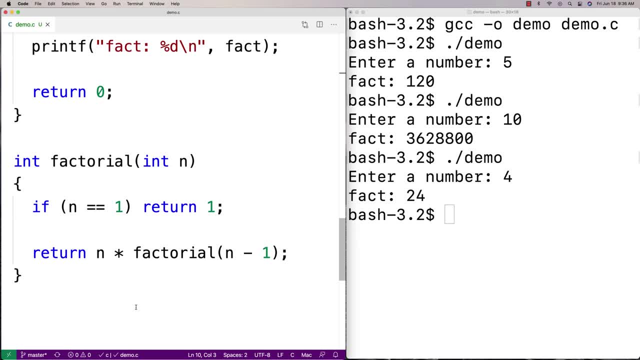 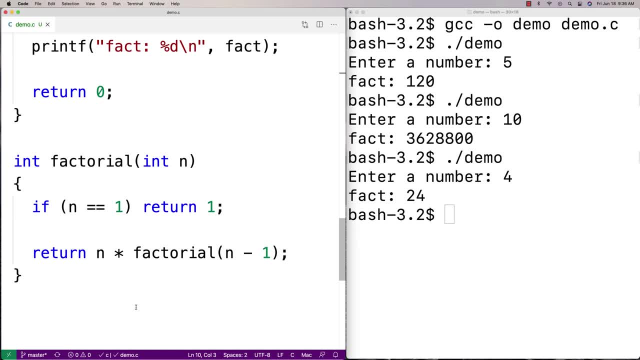 particular kind of memory it needs to call these functions. So recursion isn't a cure-all for all problems, but for certain problems, especially related to things called data structures and algorithms, recursion can actually be a great solution, because it really expresses the problem in a way that's easier to comprehend. Check out PortfolioCoursescom, where we'll help you build. 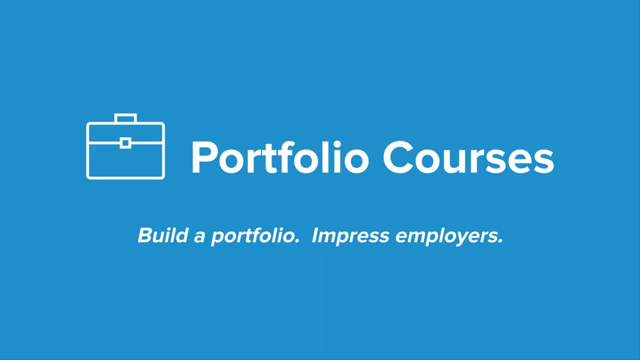 a portfolio that will impress employers, including courses to help you develop C programming projects. 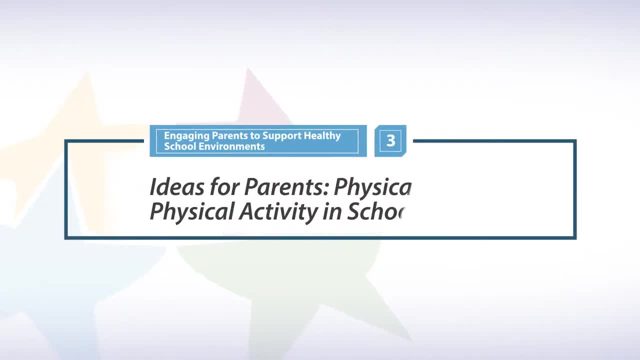 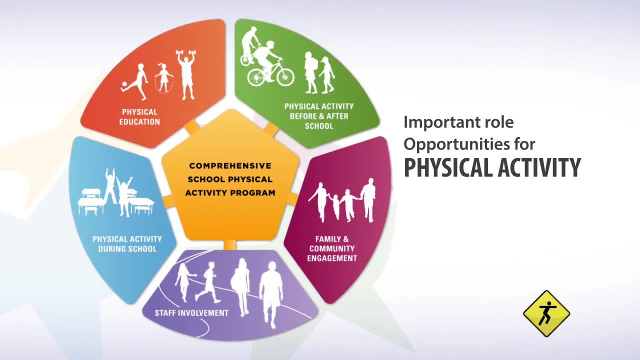 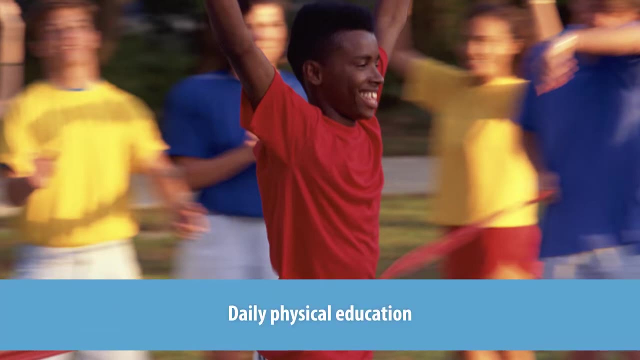 Parents can play an important role in getting schools to provide opportunities for physical activity before, during and after the school day. Examples of these opportunities include daily physical education, recess, classroom physical activity, physical activity clubs and intramural sports. Parents can help by participating on the team or committee for 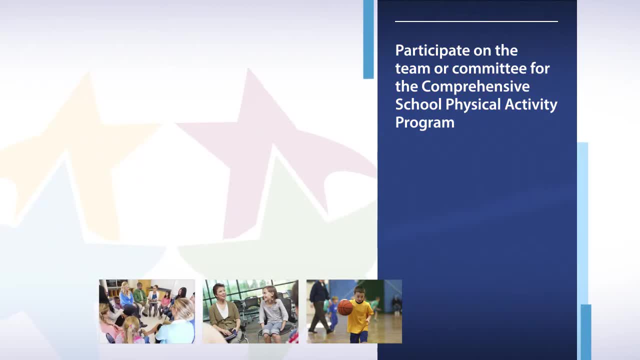 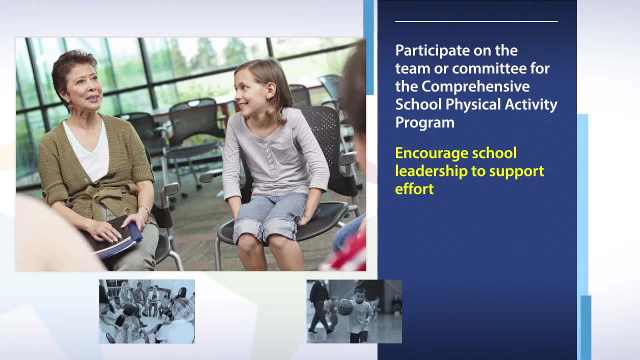 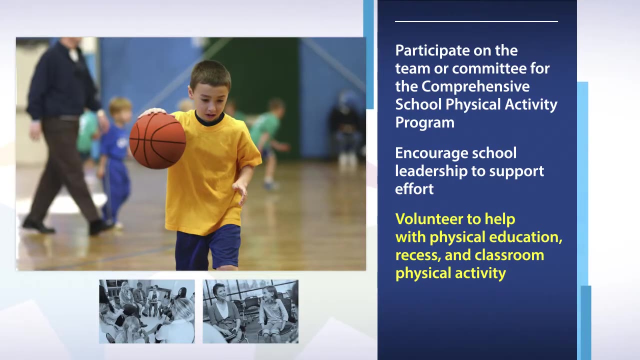 the comprehensive school physical activity program and they can encourage the school leadership to support this effort. They can be the voice at school board meetings and school health council meetings. Parents can also volunteer their time to help with physical education, recess and classroom physical activity. Parents can offer to help with activities. 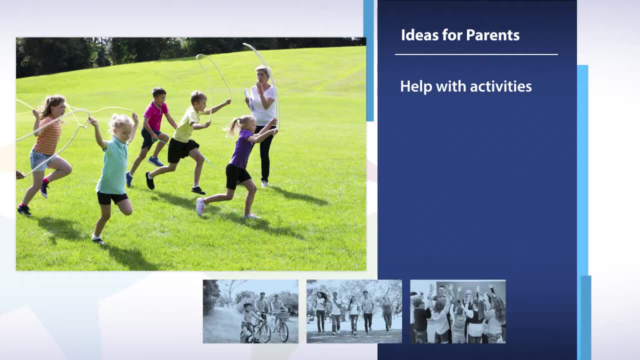 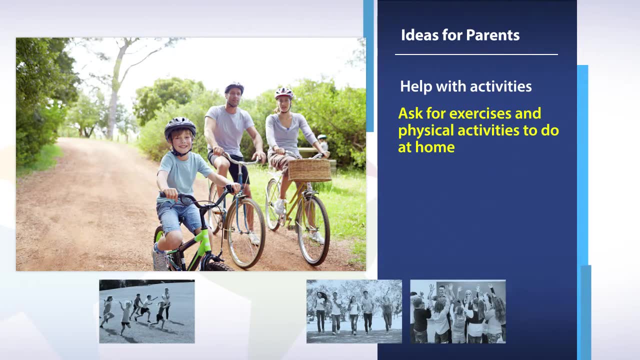 such as special physical activity programs, field trips and the annual field day. They can also ask the physical education teacher for exercises. They can also ask the physical education teacher for exercises and physical activities to do at home with their children to keep up or improve fitness levels In the classroom. 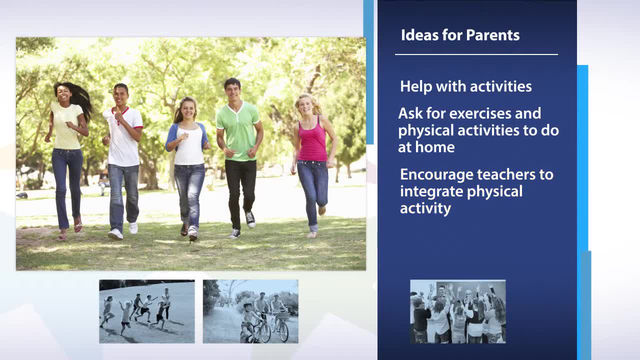 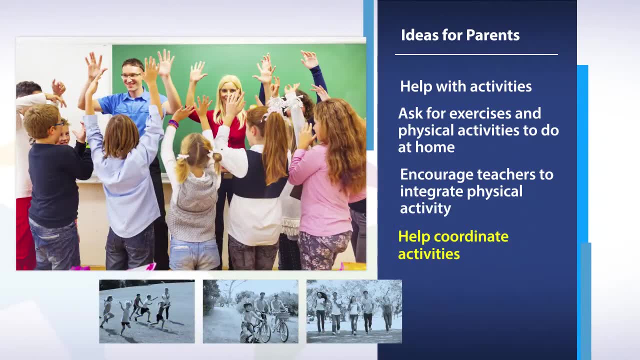 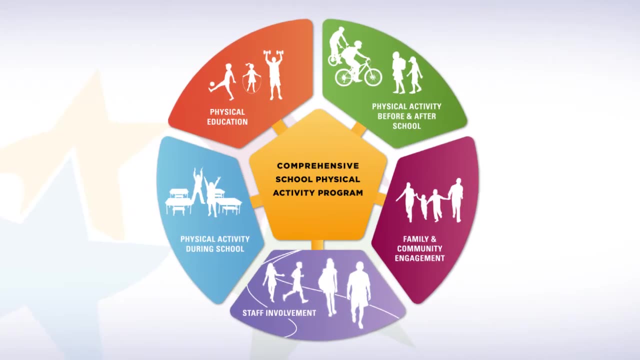 parents can encourage teachers to integrate physical activity into planned academic lessons and provide short breaks of physical activity, and they can offer to help coordinate some of these activities. These suggestions align with a comprehensive school physical activity program and can help contribute to the recommended 60 minutes of physical activity students should.